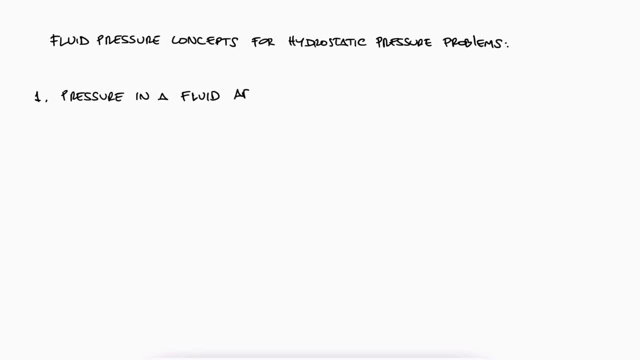 The first one is that the pressure in a fluid, in any direction, is the same. If we have any type or shape of fluid element, we would see that the pressure vector P, in any direction, has the same value. If we take a triangular element and we only use this shape so that 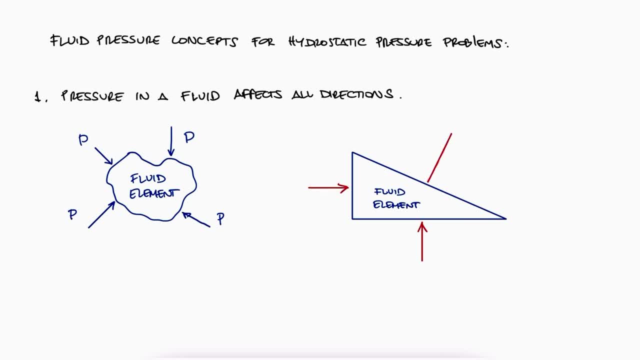 we can relate one vertical, one horizontal and one slanted pressure vector at the same time. we can prove this fact very easily. Now, if you're coming from a statics or mechanics of materials course, you're probably familiar with a coordinate system that has the x, y and z axes in this. 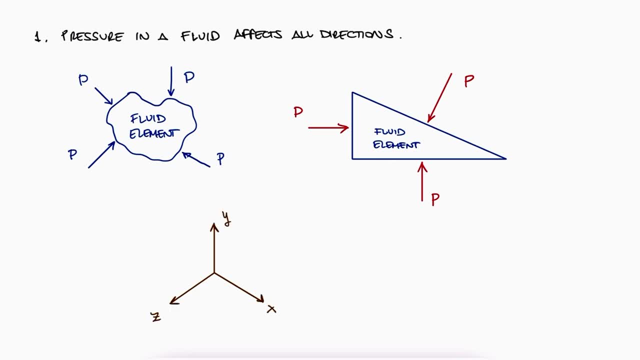 configuration, Since in fluid mechanics people usually use the z-axis for height and later concepts like head. they usually use the z-axis for height and later concepts like head and z-axis for height and later concepts like head and later concepts like height and later concepts. 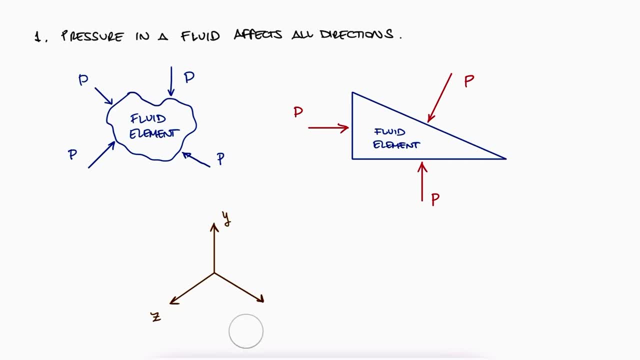 like head and later concepts like height and later concepts like height. The coordinate system for fluids usually has the x and y axes in the horizontal plane, with z coming upward. Of course, the coordinate system doesn't really matter as long as the z-axis follows the right hand rule and, more importantly, 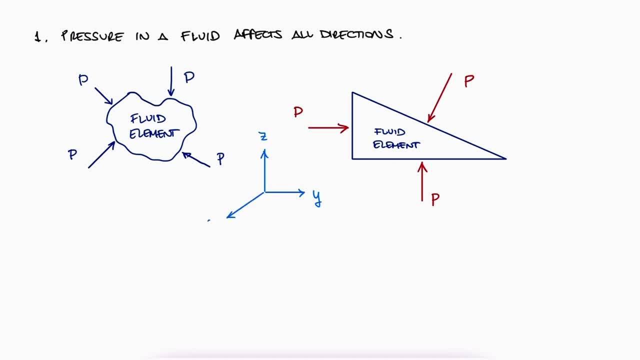 as long as you're always consistent within the same scenario With these axes. we would have some pressure vectors on this triangular fluid element on each side of the triangle and we would label them P-y, P-z and P correspondingly. The side. 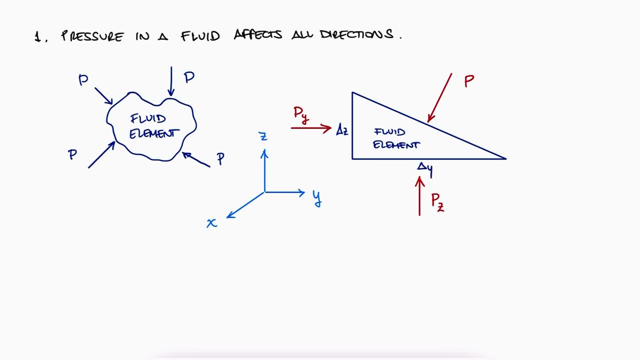 Sides would have lengths of delta z, delta y, in the third dimension not shown here, delta x and for the hypotenuse, we can call it delta s. For any triangular shape, the angle on the bottom right should just be theta. Assuming that the fluid is not accelerating in any direction, the sum of forces should: 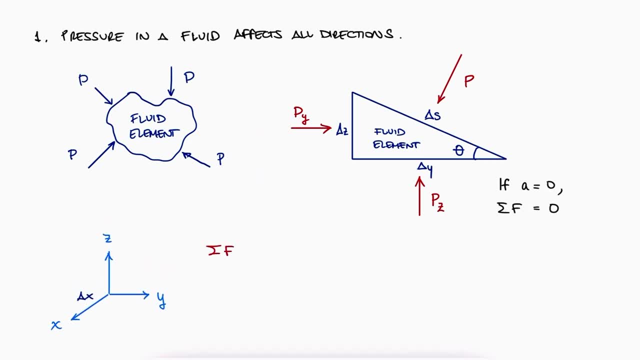 be zero. So, for example, if we do sum of forces in y, we would see py going right times the area on the left which is a delta z times delta x, and then the component of p, that is p times sine of theta times the area delta s times delta x going left. 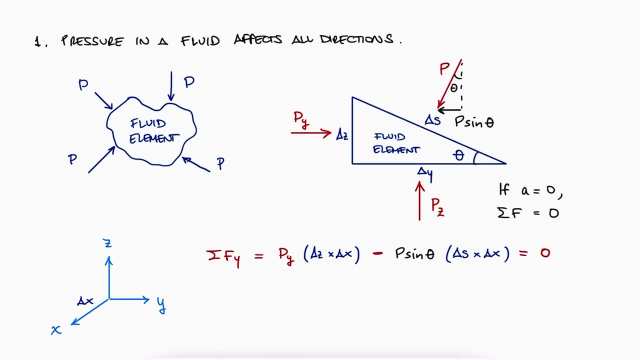 And of course this should be equal to zero again, since the fluid is not accelerating in the y direction. Since delta z can be written as the component of delta s or delta s sine of theta, we see that py has to be equal to p. 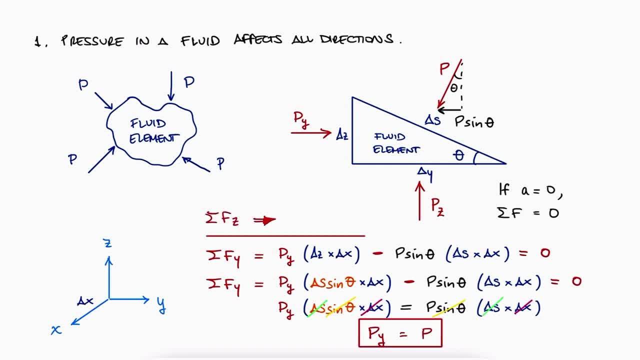 If you were to do the same with the sum of forces, sum of forces and z, you would get that pz also has to be equal to p. And notice that this is true for any angle. theta, which means that the pressure in a fluid is indeed the same no matter in which direction. 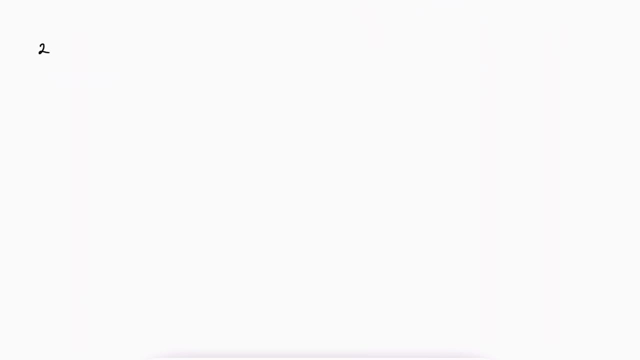 This is what we call Pascal's Law. Now, the second concept is that the hydrostatic pressure- which does not necessarily mean water, despite the hydro prefix- increases with depth inside a fluid For an infinitesimal fluid element. dzdy, we can write it as delta z times delta y. 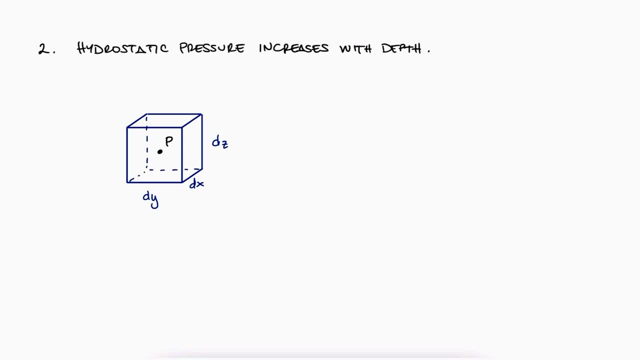 dx that has a pressure p right in the middle, We can write the pressure values for the pressure vectors on its sides in terms of p and their changes in pressure with respect to each direction or, what is the same, the pressure derivative. 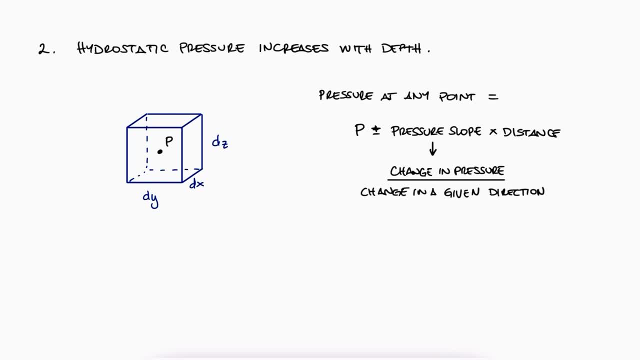 with respect to each direction. This means, for example, that for the right face we have a pressure p plus, however much the pressure has changed in the y direction when advancing a length equal to dy over 2. It would be the same, except for a negative sign. 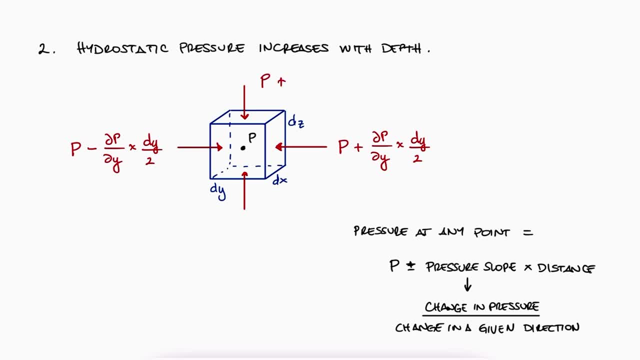 This is the same, but with the z-terms on the top and bottom faces. Each of these times, the area they are affecting would be the force values. Remember force is equal to pressure times area. Additional to these forces and the ones in the x direction not shown here, we would have: 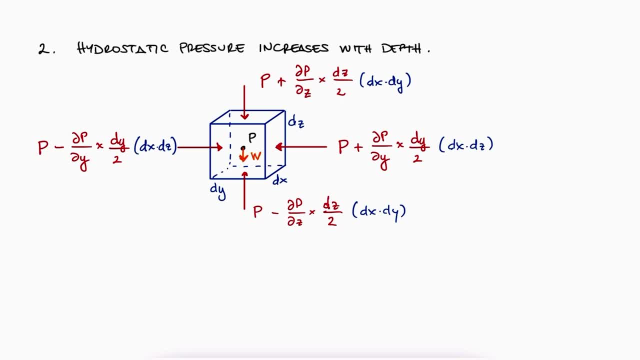 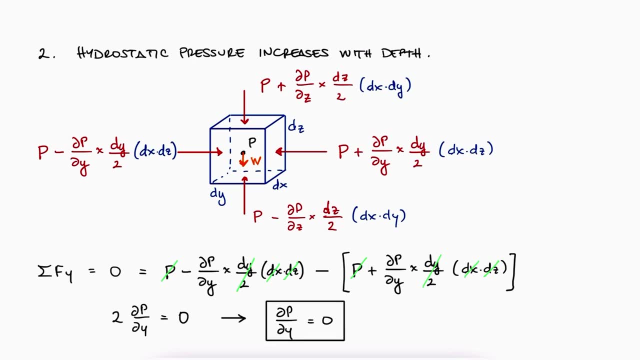 the weight of the fluid element. Therefore, for sum of forces in y, for example, we would get that the partial derivative of p with respect to y is zero When we do the sum of forces coming in and out of the screen, meaning sum of forces in. 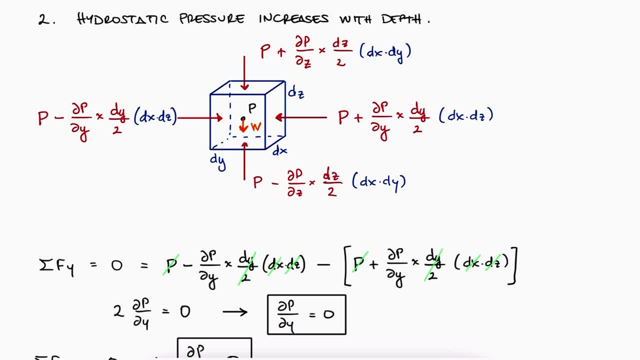 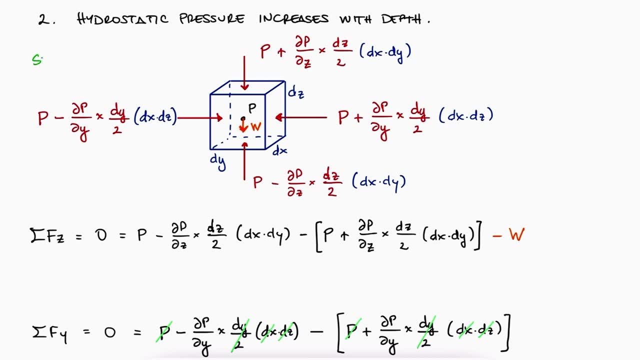 x, we would get the same for partial x of p. However, when we do the sum of forces in z, we're going to find the weight of the fluid element itself, If we use the specific weight property that we talked about during the last video, gamma. 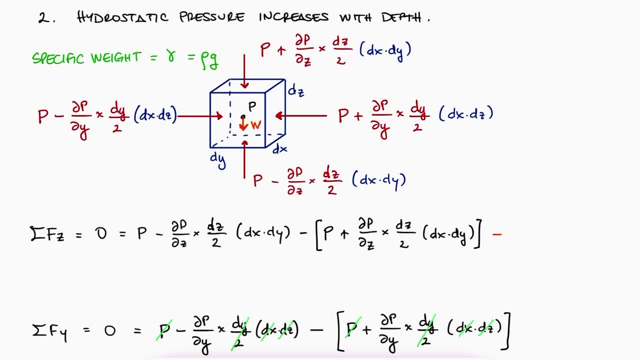 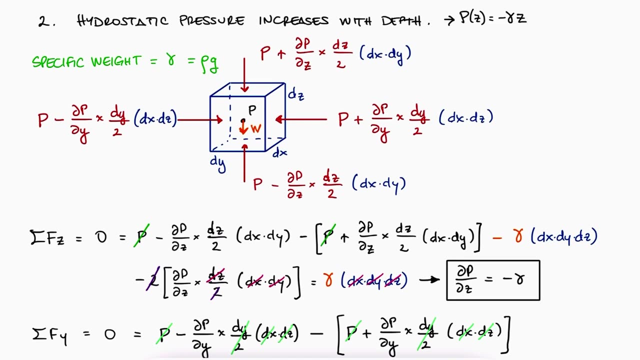 link below. the weight can be written as: gamma times the volume of the element, dx times dy times dz. Solving for partial z of p, we see that the change in pressure in the z direction is equal to the negative value of gamma or, what is the same, that the pressure increases when. 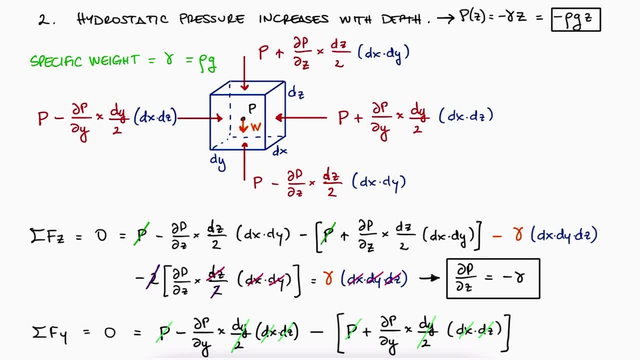 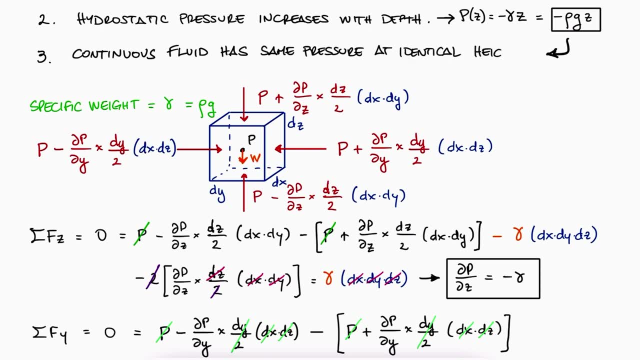 we go deeper Tied to this conclusion. the third concept we'll cover is the fact that the fluid pressure is the same at the same height value as long as we don't leave the fluid or cross any solid barriers. If we have a pressure p at this location and we move up or down, the pressure is going. 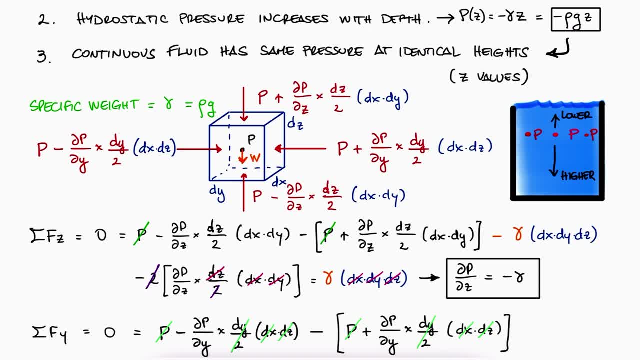 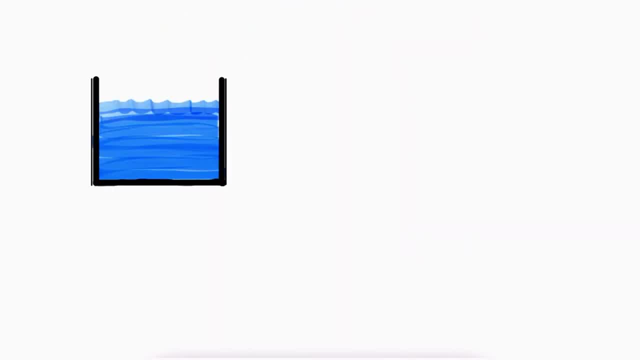 to change. but if we move left or right, or into or out of the screen, the pressure is the same And this makes sense. If we had different pressure values for the same fluid in two different locations that share the same z position, we would have an overall force going from the higher pressure. 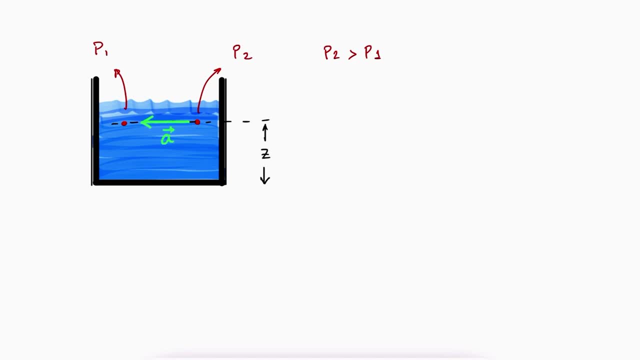 value to the lower one, causing the fluid to accelerate in that direction. And this is also true if we're looking at a continuous line of liquid, even if partially separated by a wall or contained within a tube. If the pressure was higher on one side than the other, the fluid would be accelerating. 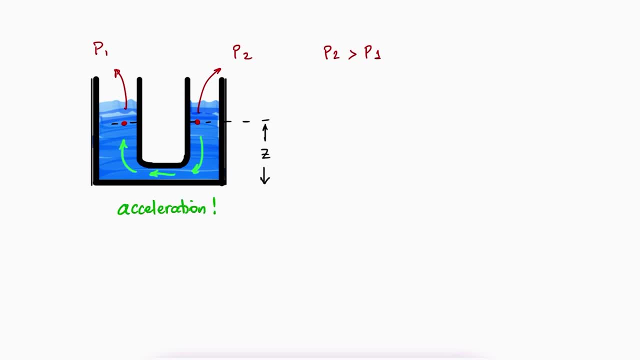 towards the lower pressure direction, And this makes sense. Before we quickly go over some examples to better understand this concept of a continuous fluid, we'll point out the difference between absolute pressure and gauge pressure. The atmospheric pressure is the pressure of air, a fluid, of course, at sea level. 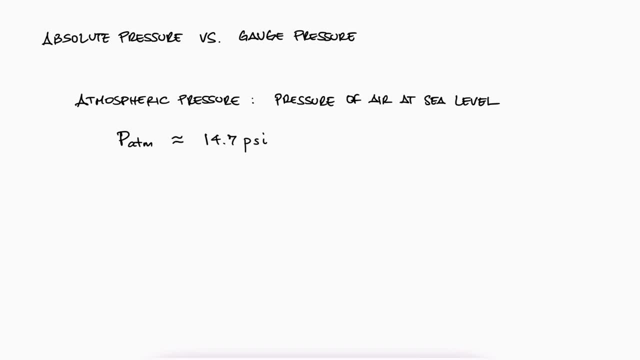 This value is about 14.7 psi, 1001,325 pascals, 1013 millibar, 760 millimeters or 29.92 inches of mercury, And the atmospheric pressure is the pressure of air, a fluid, of course, at sea level. 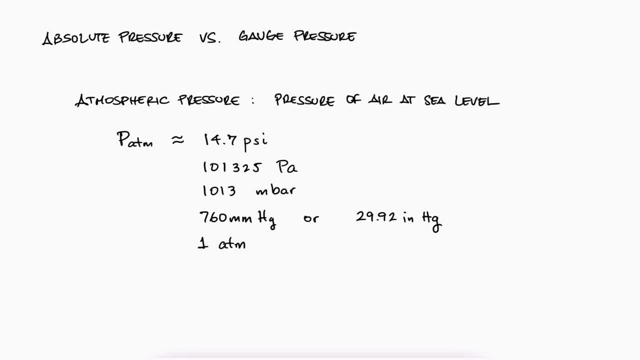 That's the same for all the other pressure values. Of course, depending on the temperature and the altitude, the atmospheric pressure can change. So, for example, in a city with an altitude of 8500 feet the atmospheric pressure is about 72% of that at 73 kilopascals or 10.6 psi. And don't let weather websites throw you off by reading their mean sea level pressure, which you can learn more about in a link below. Therefore, the difference between the absolute pressure and the gauge pressure is very simple. The atmospheric pressure is about 70% of that and the atmospheric pressure is about 72%. 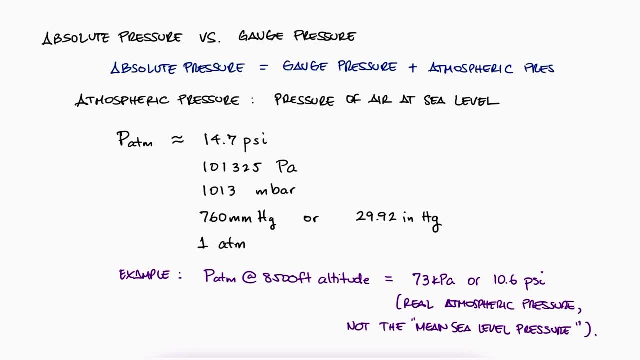 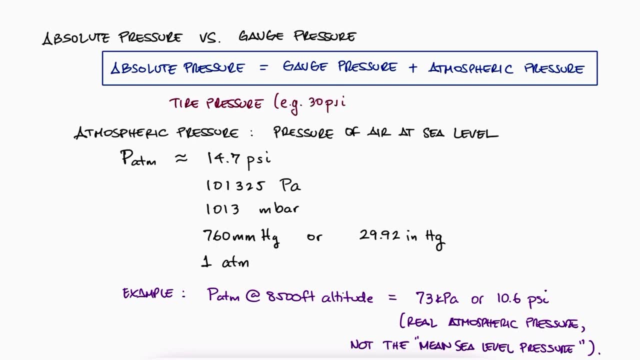 of that or 10.6 psi, But don't let weather websites throw you off by reading their mean sea level pressure. pressure is precisely the atmospheric pressure. For example, when measuring the tire pressure, we use gauge because we want to know the pressure inside it with respect to the outside pressure. 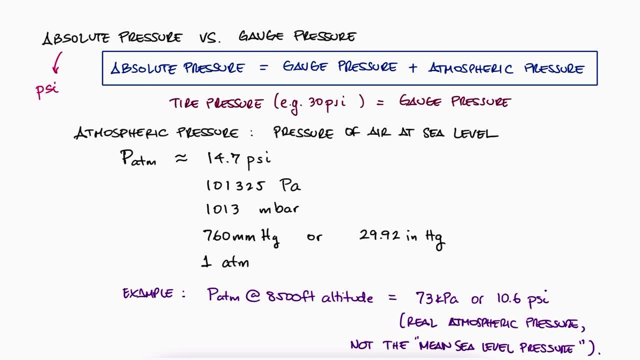 For their units. we usually label them PSI-A for absolute and PSI-G for gauge. If only PSI is used, it most probably refers to gauge pressure. In metric absolute pressure usually goes with an ABS in parentheses. for example, 120 kilopascals absolute pressure. So let's 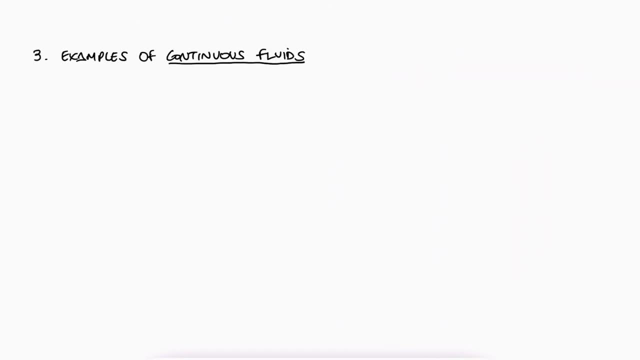 look at the examples of when pressure is equal and when it's not equal. Let's say there's water with specific weight 1, in a reservoir that has a wider opening on one side than the other, Regardless of the horizontal cross-section area or, in this 2D representation, the width. 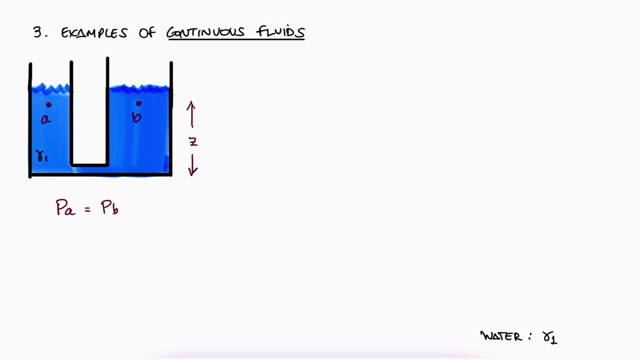 the pressure is the same at A and B. Remember that the pressure is not a function of the area or anything else, it's just the pressure. If we now close one side and put some pressurized air in there so that the free surface that 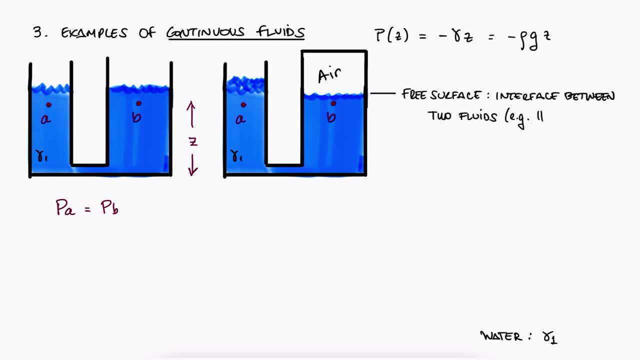 is the interface between two fluids, in this case water and air, is lower on that side. the pressure is still the same at A and C. We could even bring these points closer to the free surface to find out that the gauge pressure of the air in the closed space is. 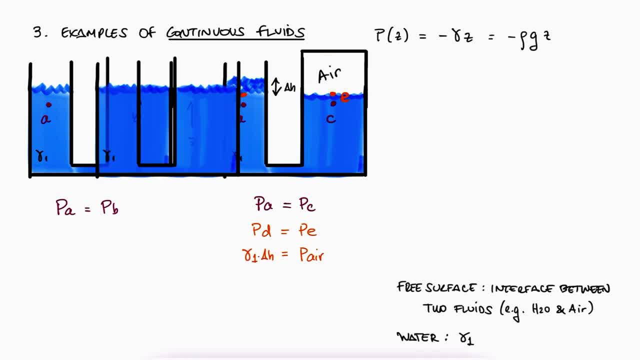 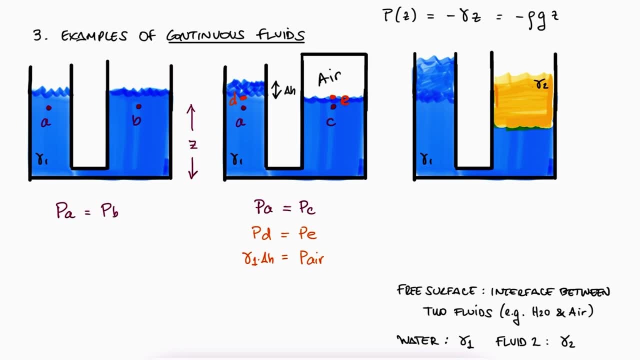 equal to gamma 1 times delta H. Now let's say that the right side is open again, but this time we throw in a C. This time the pressure in A and the pressure in F would not be the same. Why? Because to 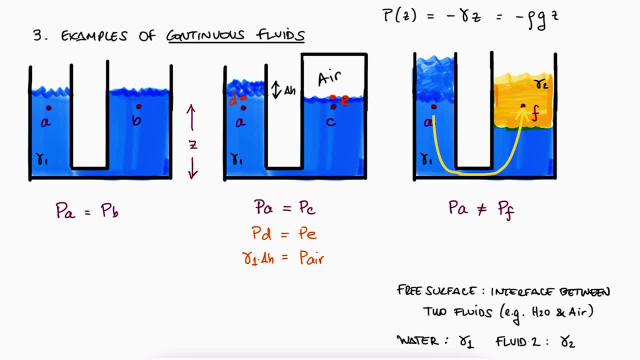 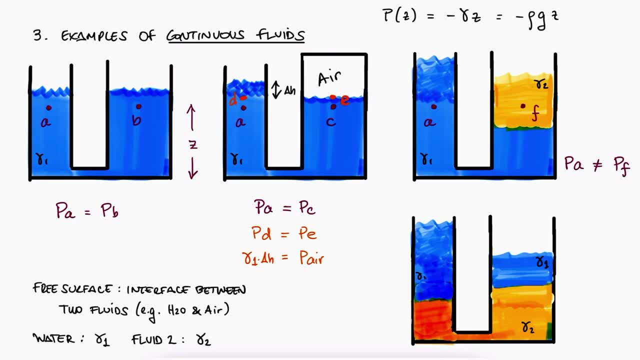 get from A to F, we had to jump away from our original fluid, Even if we end up on the same fluid, in this case water, meaning we start with water and end with water if the fluid is not continuous. if we had to jump between fluids to get from one point to the 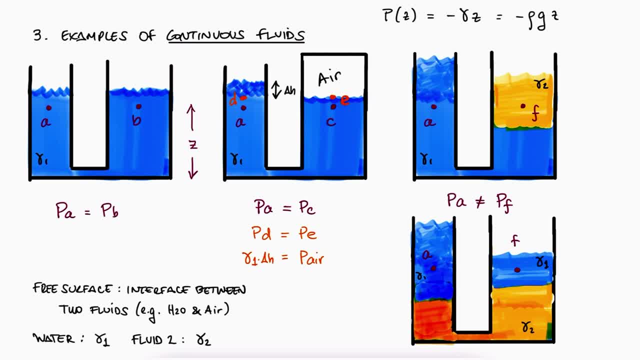 other, we cannot state that the pressures are the same. However, if we lower the air pressure, the pressure is still the same, and if we lower the original location of our two points, then, yes, we can state that the pressures are the. 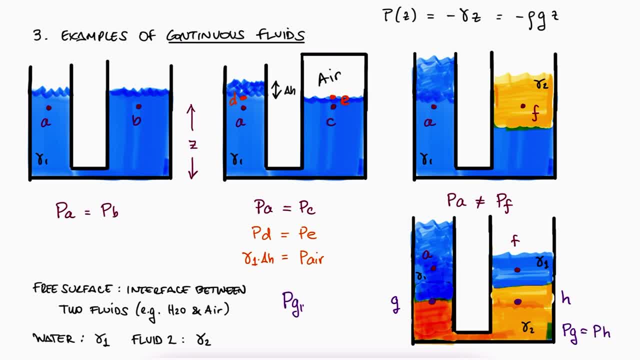 same And again. this can be useful because the pressure at G in the water and the pressure at G in the second fluid are indeed the same. More on that in just a second. Finally, if there's a solid division in our reservoir, even if we have the same fluid, 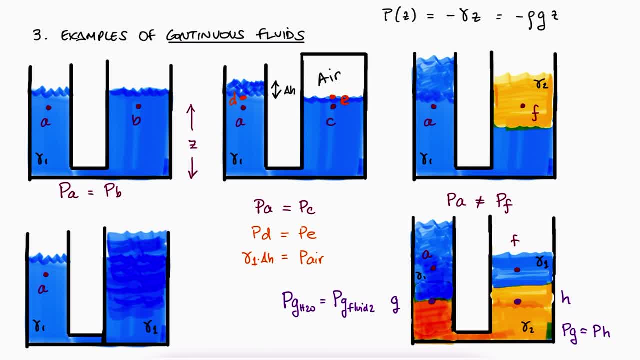 we cannot guarantee that the pressures are the same, even if they are the same fluid, because, again, we had to jump over a solid obstacle, meaning the fluid is not continuous. Alright, let's look at an actual example where we use this to find the pressure inside. 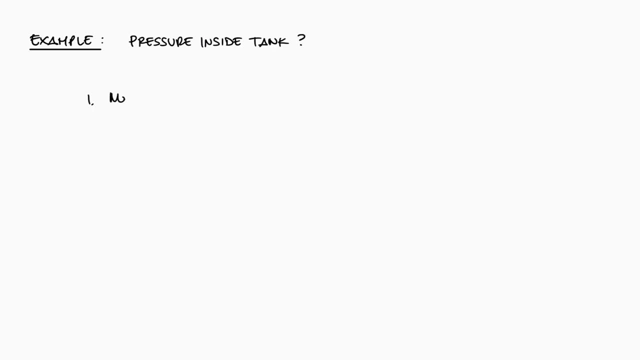 a container. If you want to check out other more complex examples, the other lectures of the fluid mechanics course or even lectures from other engineering courses like mechanics of materials or machine design, make sure to check out the links in the description below. Let's say we have a water tank pressurized by air. We connect an oil and mercury manometer. 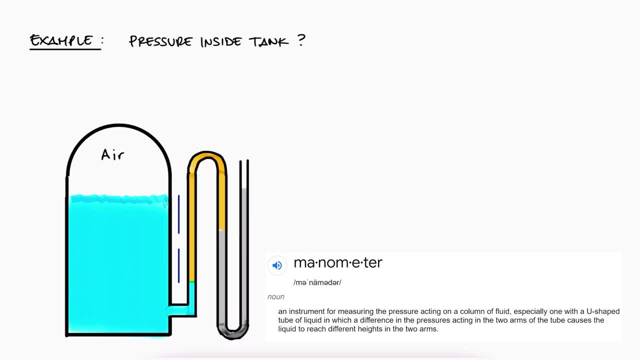 to measure the air pressure inside the tank, Knowing the values for the height of the liquid liquid columns and the density of the fluids. what is the air pressure inside the tank? From what we learned today, we know that the pressure at A is the outside pressure plus. 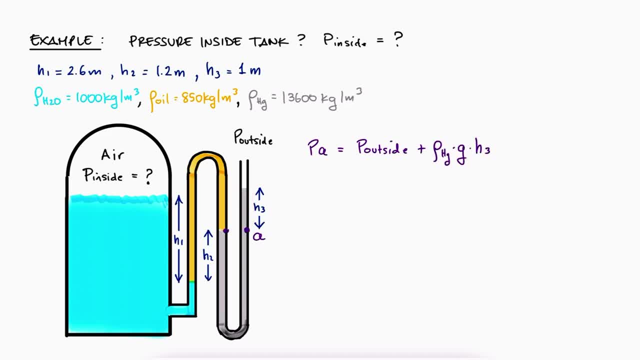 the column of mercury. And if we go from A to B we are in the same continuous fluid and therefore PA and PB are equal. PD is equal to PC plus the column of oil. but again PC and PB are the same And since PE can be written as P inside plus the column of water, we can: 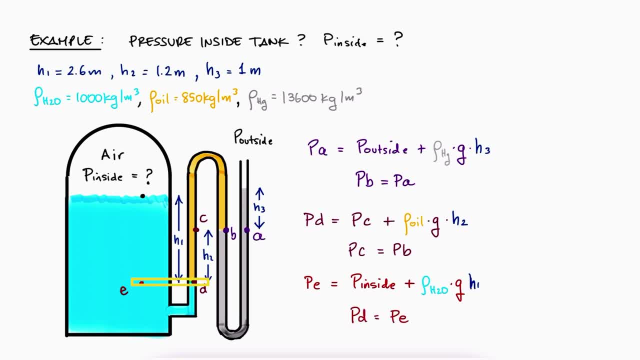 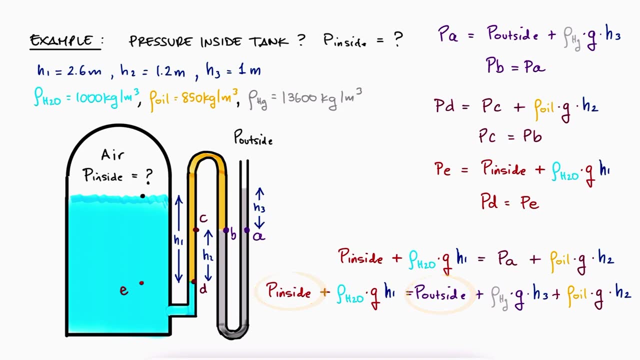 substitute PE for PD, which is already in terms of PC or PB or even PA, to obtain an equation that relates the inside pressure with the outside pressure. Alternatively, we just start at P outside. add a column of mercury add, since we're moving. 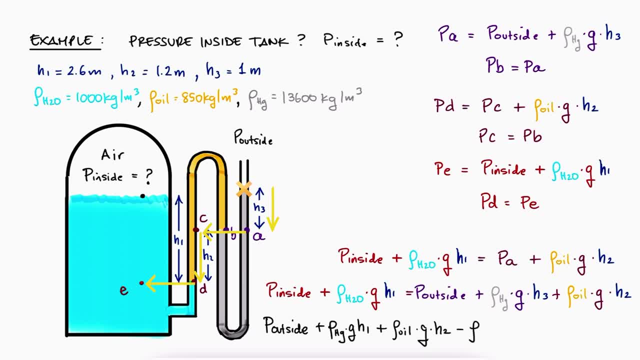 downward. add the column of oil and subtract the column of water- subtract since we're moving upward- and add the column of mercury. We can substitute PE for PD, which is already in terms of PC or PB, or even PA, to obtain an equation that relates the inside pressure. 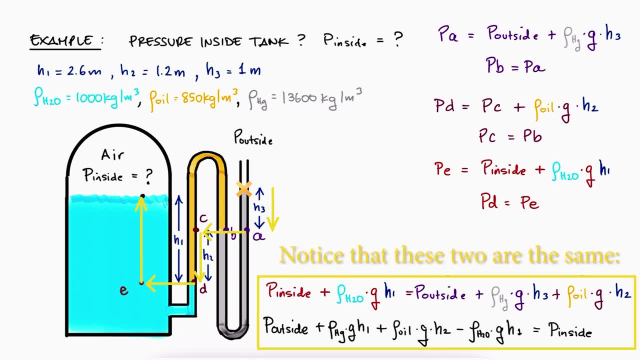 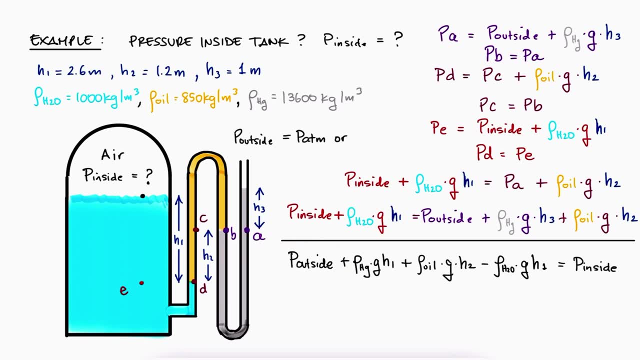 to find P inside. With this we can either find the absolute pressure inside the tank, if we say P outside is the atmospheric pressure, or we can find the gauge pressure inside the tank, if we say P outside is zero. Regardless, we substitute the values and find the pressure. 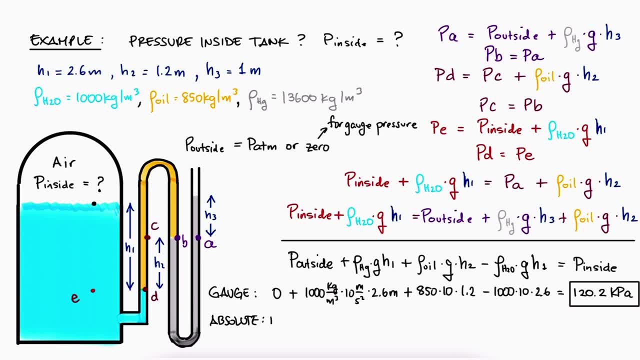 to be roughly 120.2 kilopascals or 221.5 kilopascals. Don't forget to check out the links in the description below for more examples, more lectures or any other questions. Thanks for watching.